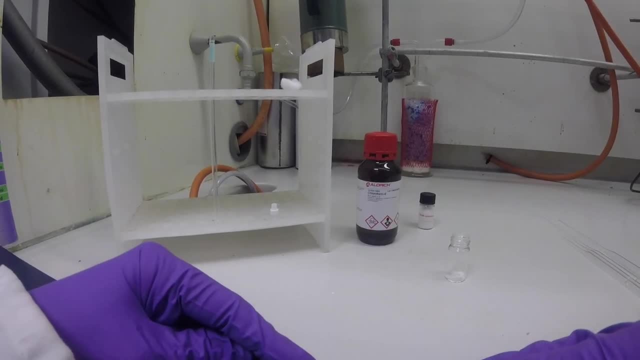 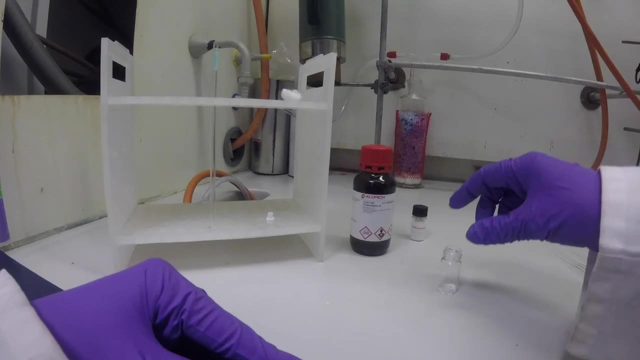 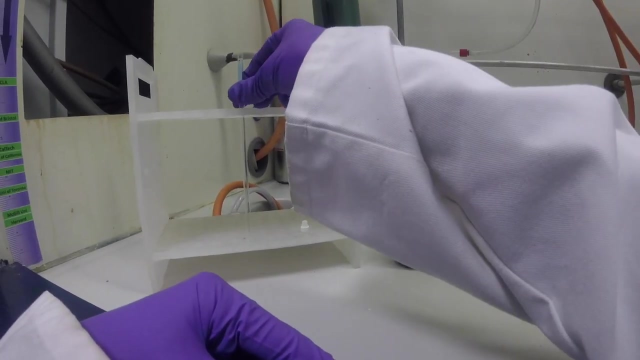 In this video I'm going to show you how to make an NMR sample. Before you start making your NMR sample, it's good to have everything you need to hand. So here I have my compound of interest: some deuterated NMR solvent, an NMR tube, an NMR lid, some pipettes and 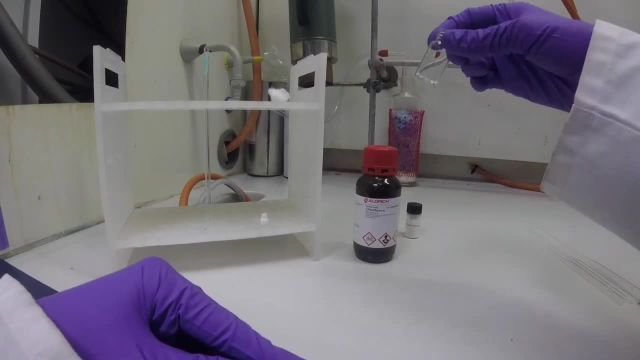 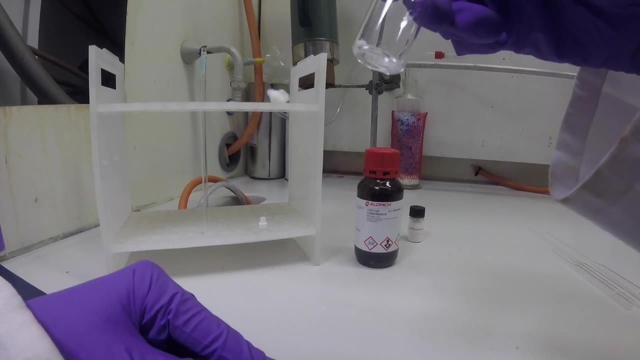 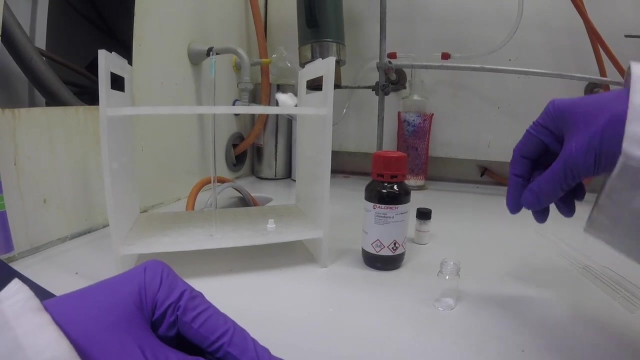 cotton wool for filtering NMR is quite an insensitive technique, so we need to have quite a large amount of sample: a couple of mgs for a proton NMR and maybe about 20 mgs for a carbon NMR. The first thing we need to do is dissolve up our sample. I'm using deuterated 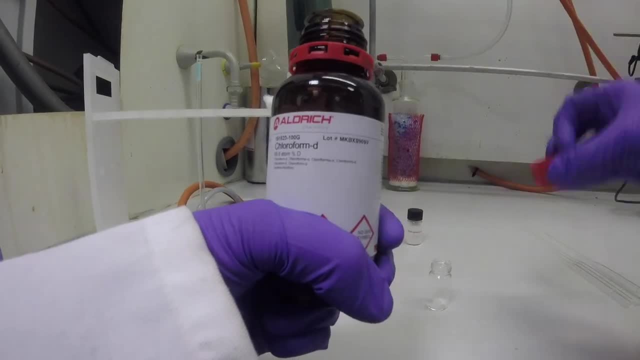 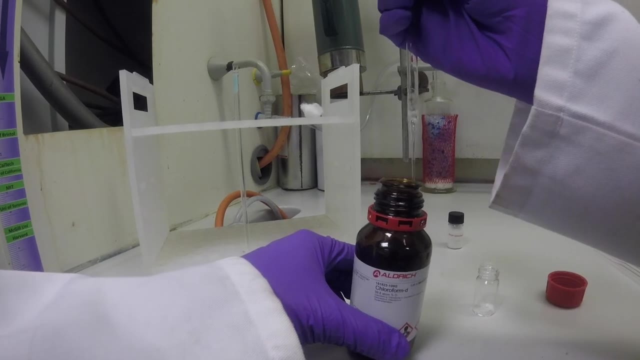 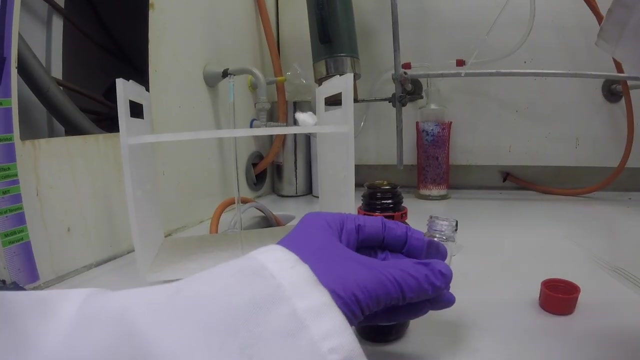 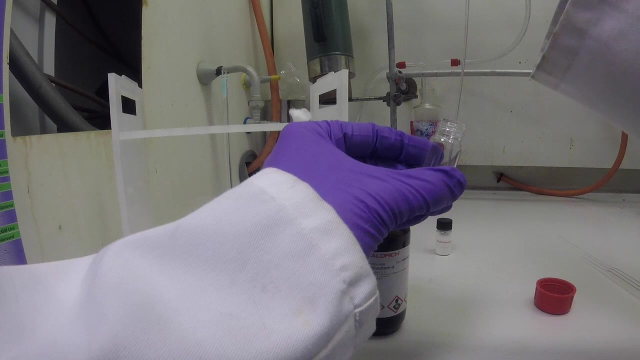 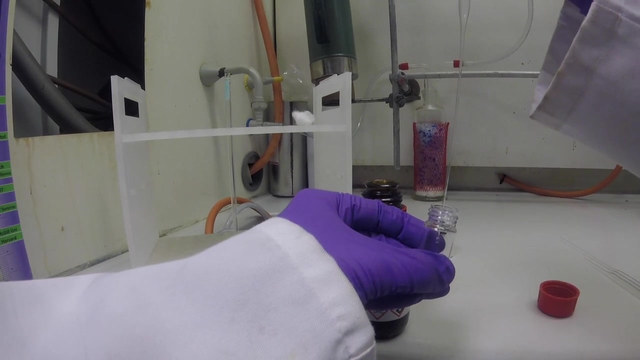 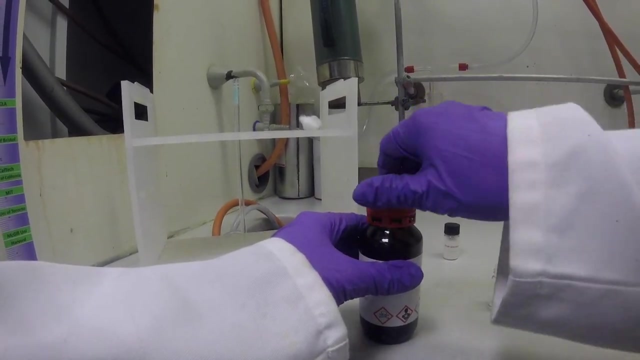 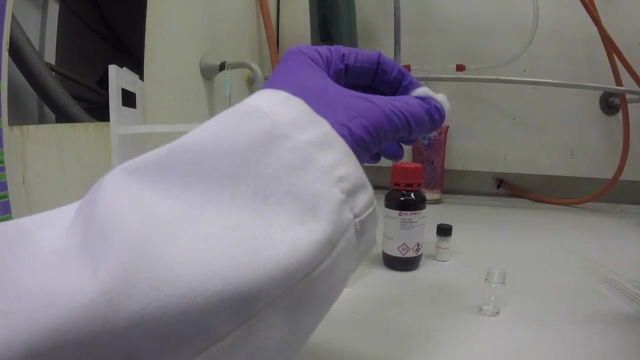 chloroform and you need to use about 0.7 ml of solvent. This should give you about 4cm of depth in your NMR tube. Make sure your sample is mixed OK, OK. OK OK. In order to filter your sample, you need to pop a small amount of cotton wool into a short. 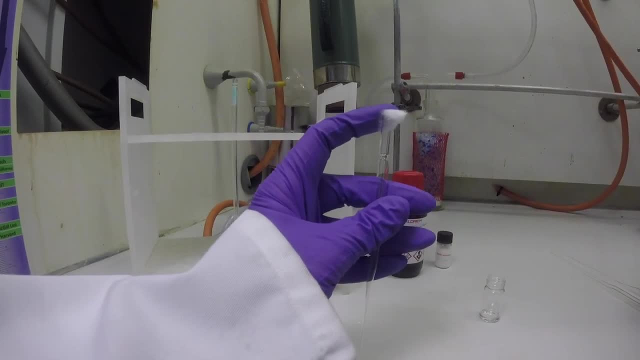 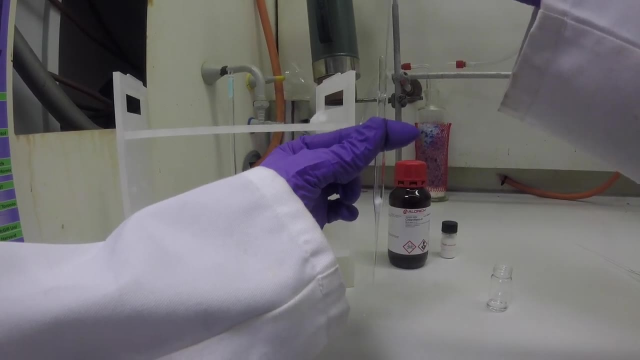 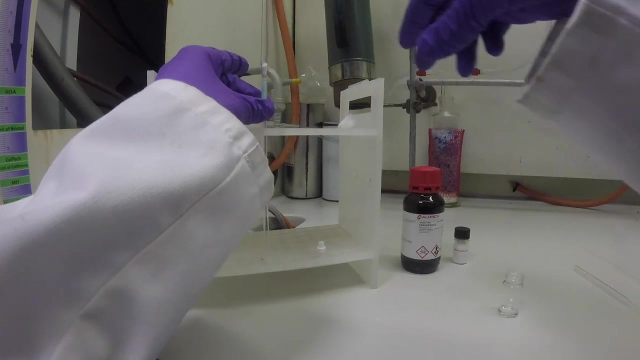 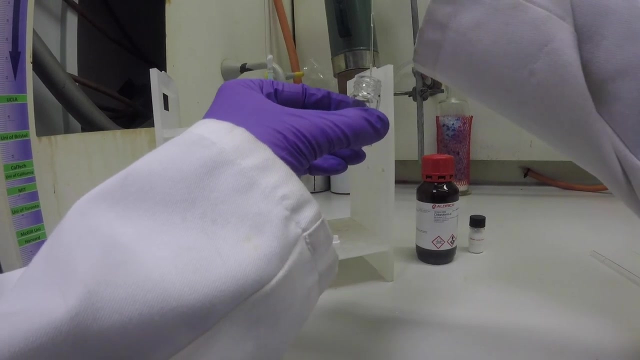 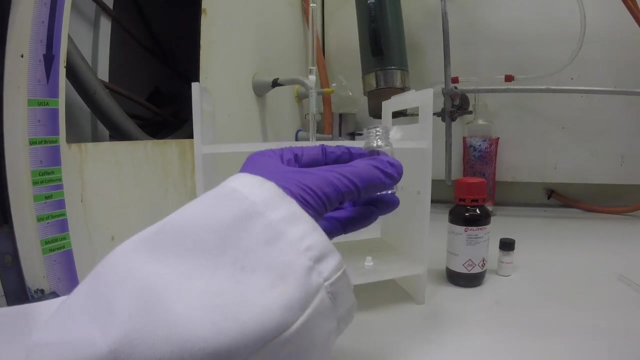 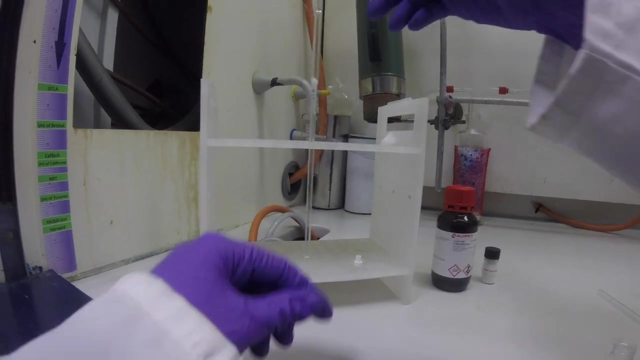 pipette. It's useful to use a long pipette to pop the cotton wool to the bottom. You can then put this filter at the top of our NMR tube. OK, OK, OK, OK, OK, OK, And add our dissolved sample. 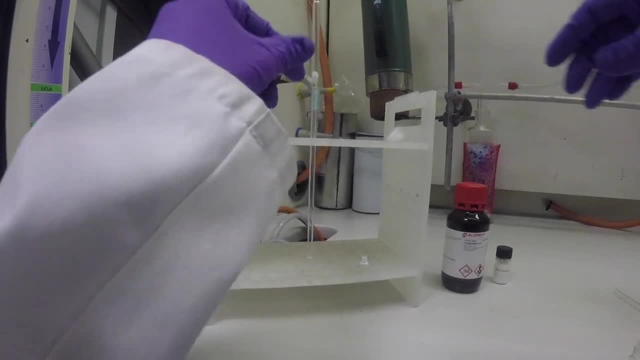 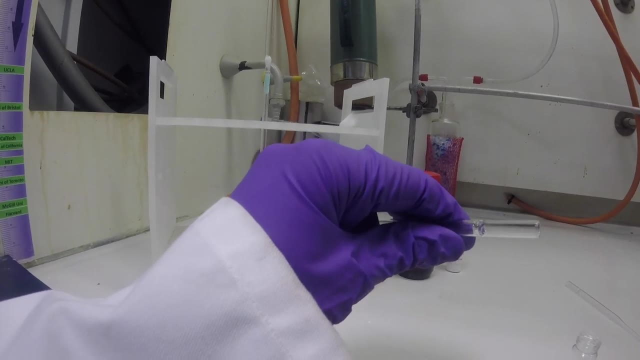 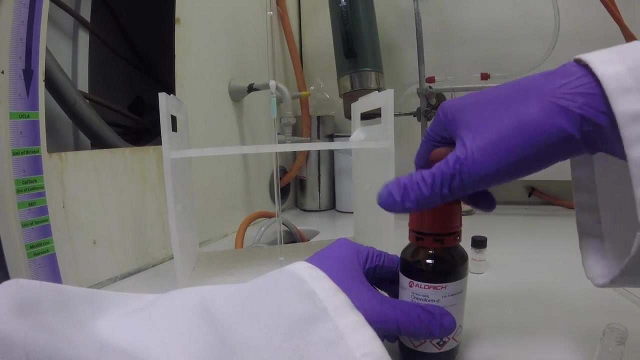 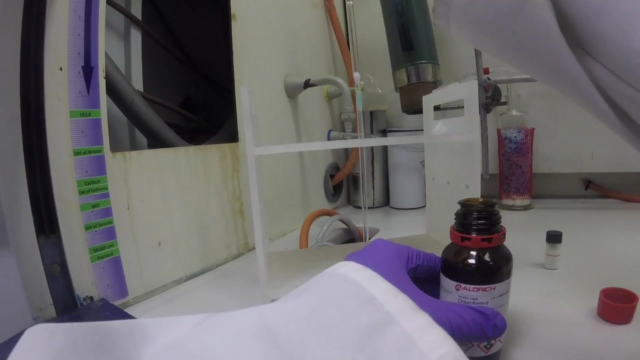 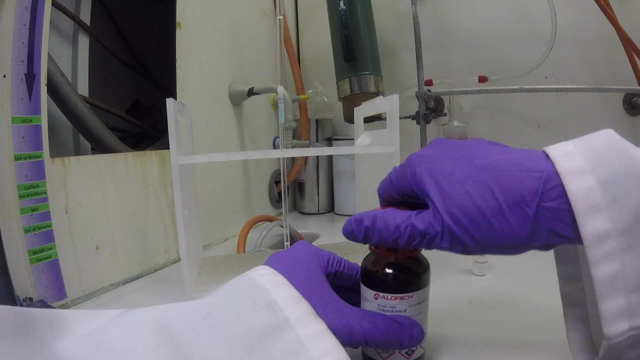 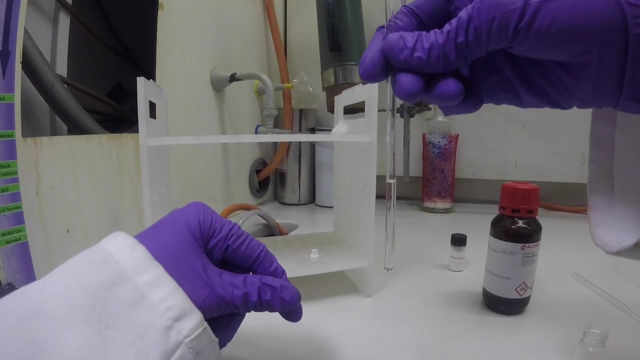 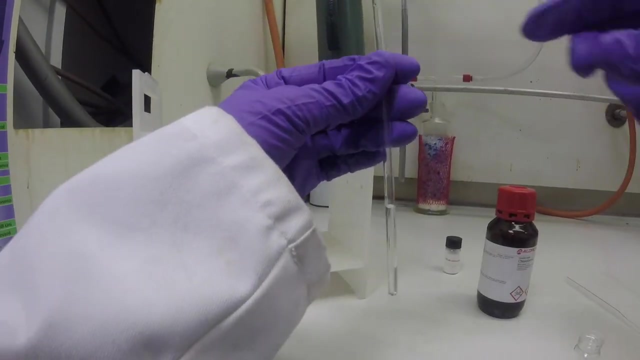 OK, OK, OK, OK, solvent. be sure to use a fresh pipette to add more and you should have your four centimeters depth in your NMR tube and we can put the lid on. lots of other people will also be running NMR samples, so it's. 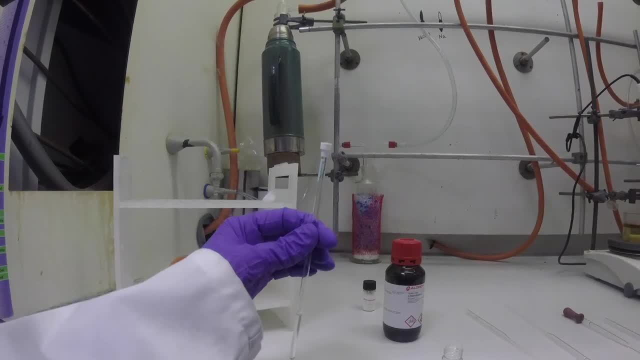 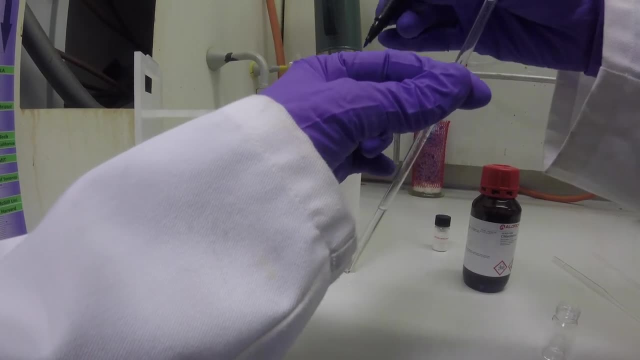 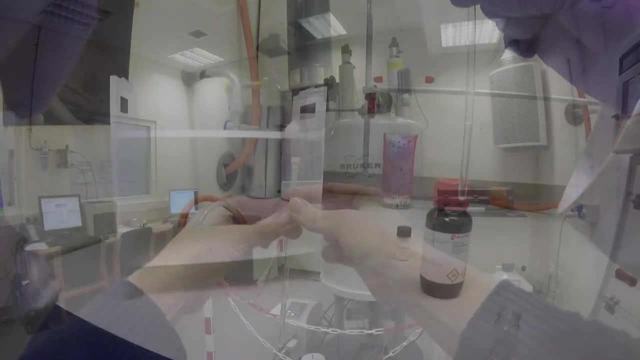 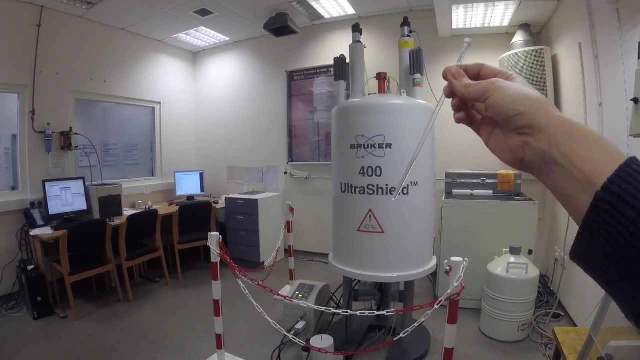 important to label your sample tube carefully. next we go to the NMR machine. so i've arrived in the NMR lab. i'm going to put my sample on the 400 megahertz NMR spectrometer that you can see here, because i added some extra solvent to my sample earlier. 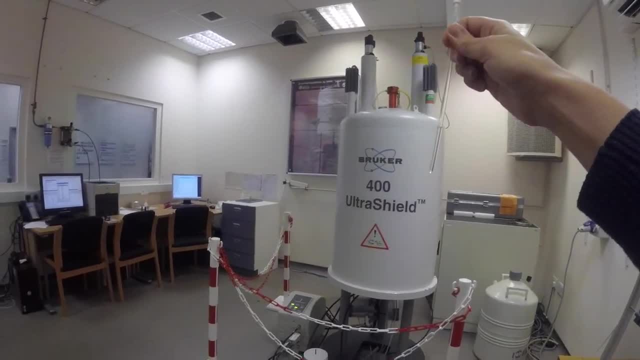 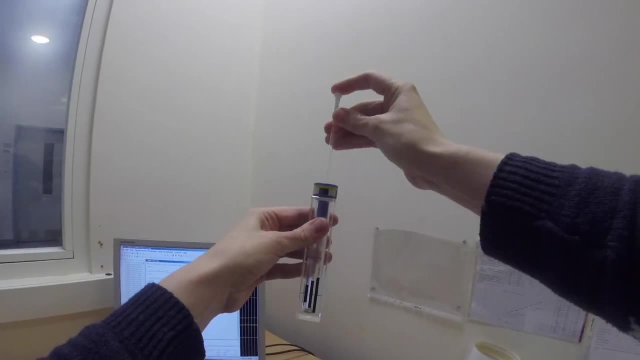 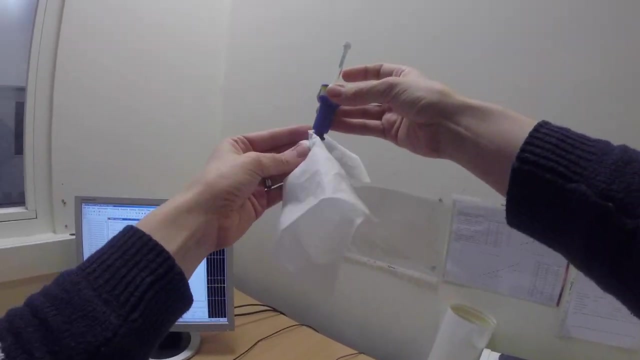 just going to make sure it's thoroughly mixed. when you arrive at the NMR machine, you need to pop your sample into a sample holder and use the depth gauge to make sure that the sample goes the appropriate depth into the probe. i'm going to give the sample a wipe for the tissue on the outside to remove. 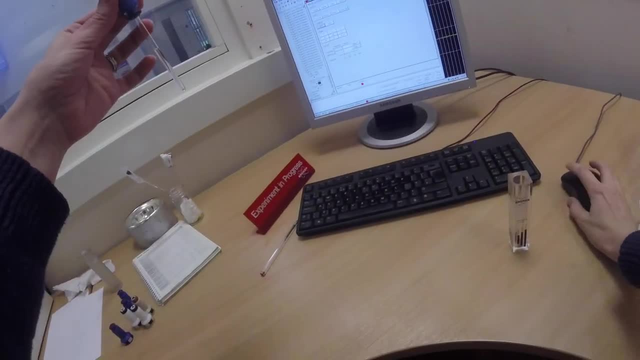 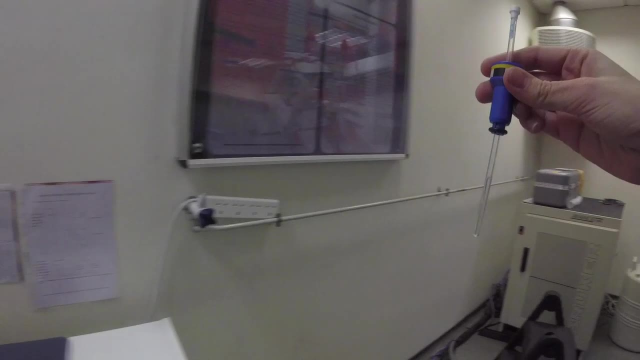 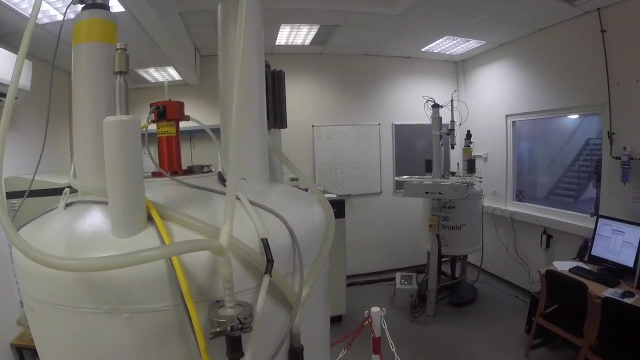 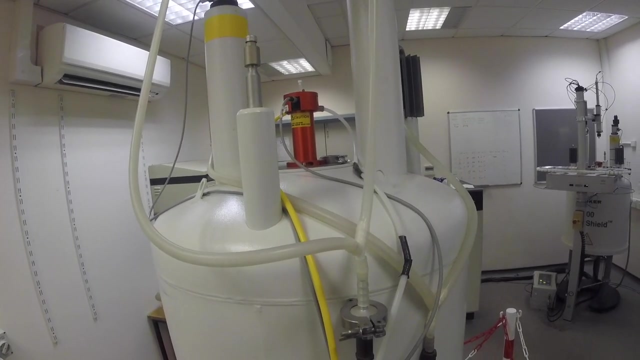 any contamination that would otherwise get into the NMR probe, and in order to lower our sample carefully into the NMR machine without breaking it, turning on a supply of compressed air such that the NMR sample hovers on the bed of air. once the sample is hovering we can turn off the air supply and it will be lowered slowly. 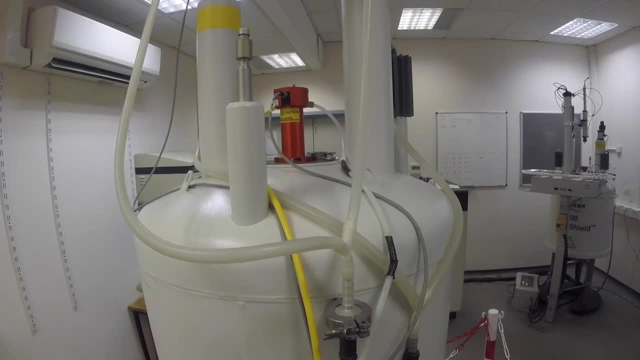 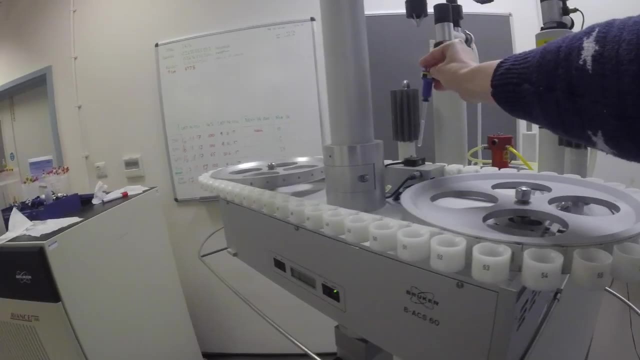 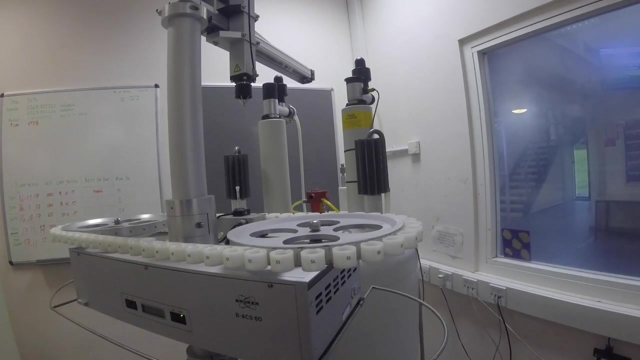 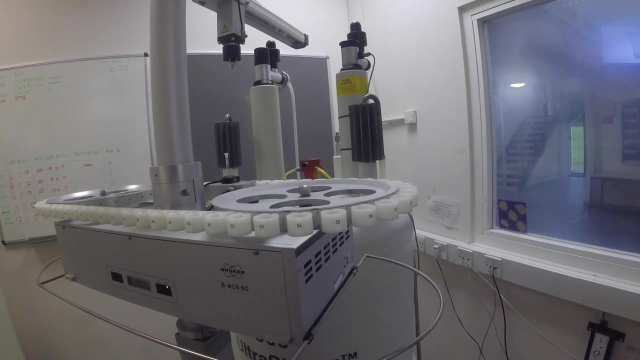 into the center of the magnet. alternatively, if you're short of time, you can use one of the automation machines. in this case, the robot arm will pick up the sample for you. all you need to do is once again tell it which experiments you'd like to run.